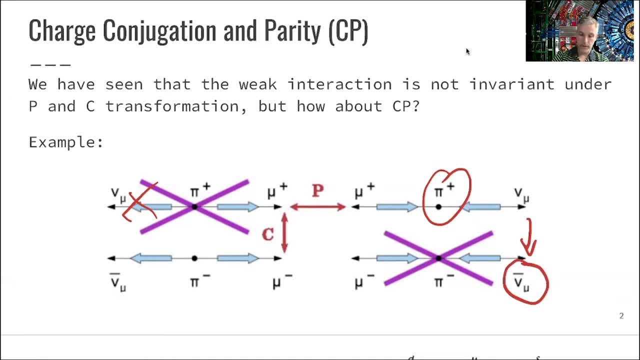 left-handed and also those two nexus in nature. So parity or charge conjugation doesn't really work on those decays, those weak decays. But what does work? if you apply the parity and the charge conjugation together, You turn the positively charged pion into a negatively 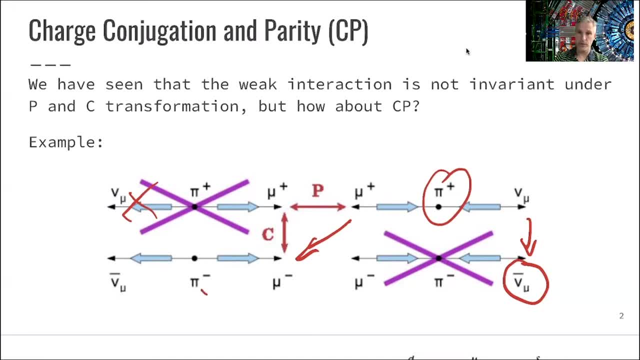 charged pion, the antimuon into muon and the neutrino into an antineutrino. So the two are connected. So you can see that the more you apply the parity and charge conjugation together, the positive charge pion becomes a negatively charged pion, The antineutrino becomes a negative. 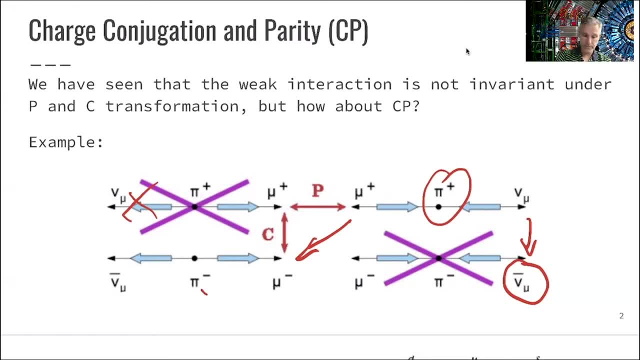 antineutrino, And you see here that the antineutrino is right-handed, So is the muon, And so that decay is actually observed in nature. Good, So we saved the day. Seems like that the weak interaction is invariant. 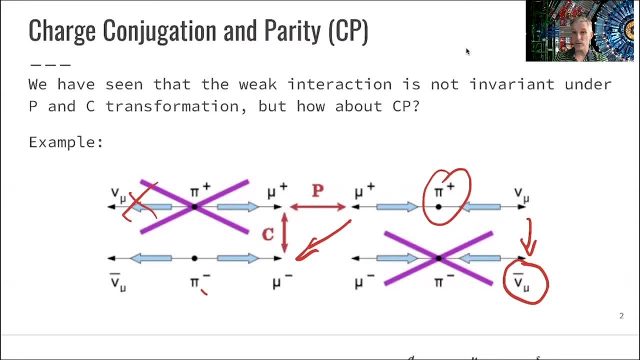 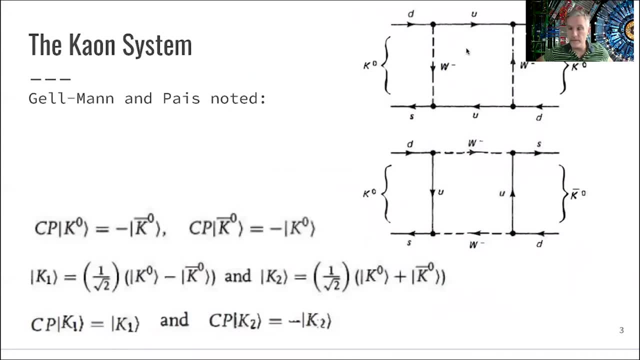 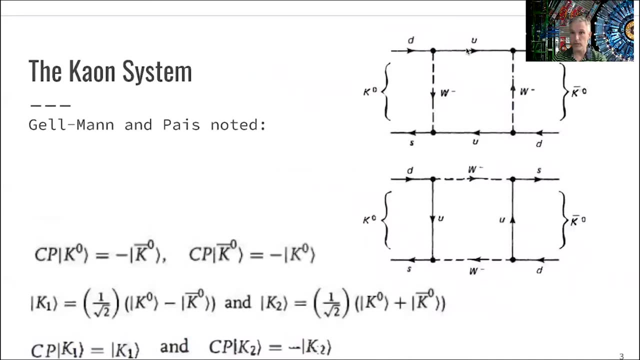 under CP transformation. However, that's not quite true. Gelman and Pace noted that in systems of neutral kaons there is an odd effect, And the effect is that a particle- a k0, can turn into an antiparticle by changing. the strangeness. 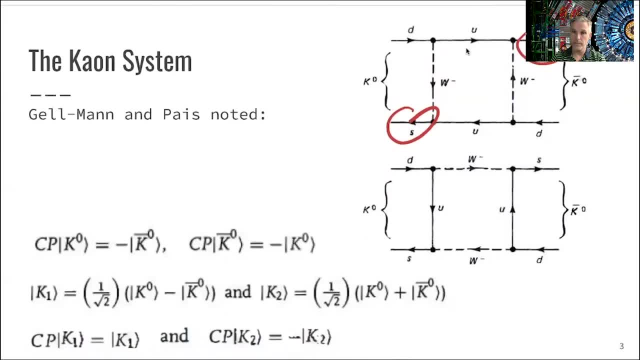 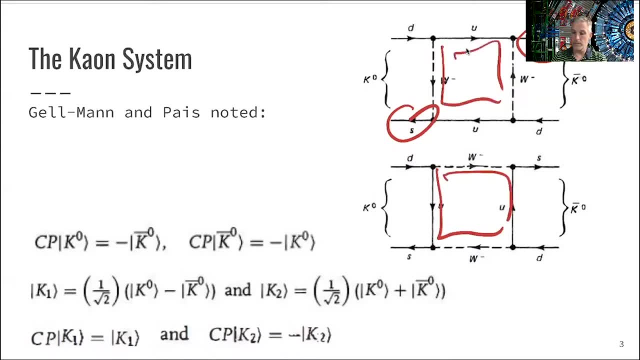 And that's possible in these kind of box diagrams which include a box with a couple of w's, And it's easy to think, It's easy to see that if you prepare a kaon it will oscillate, because those diagrams are. 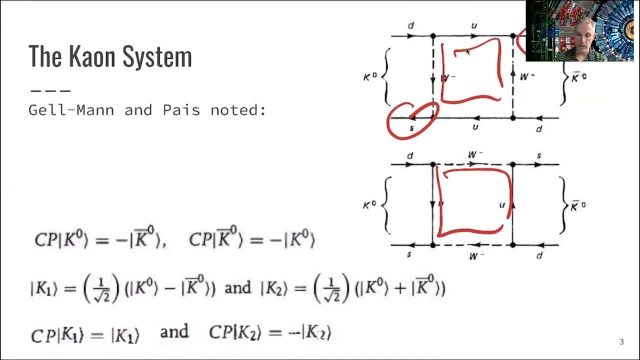 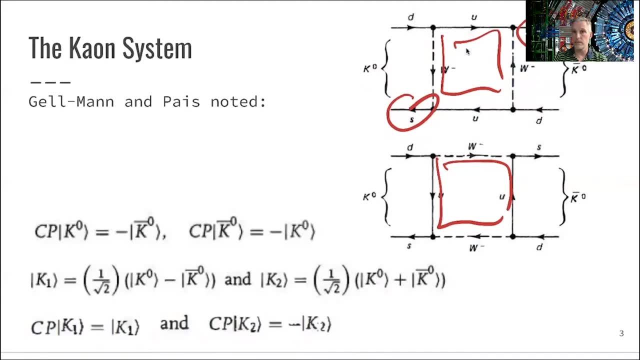 possible into an antiparticle. So now, what is happening now to CP here. If I apply CP on a kaon, I find a minus sign in an antikaon. So if you want to analyze this further, you might want to find the eigenstates to this. 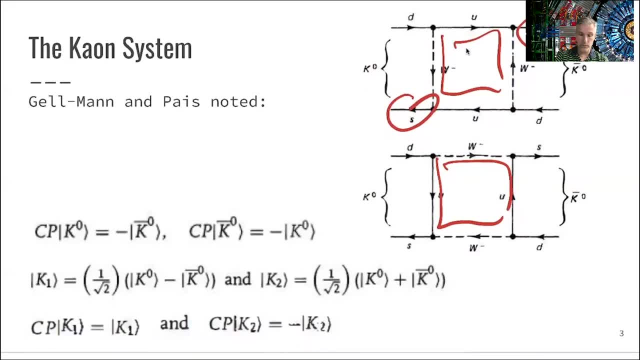 And so the eigenstates can be found as those k1 and k2, which are upmixtures of OK, Of the k0 and the anti-k0. And you find this symmetric, the symmetric and the antisymmetric states. 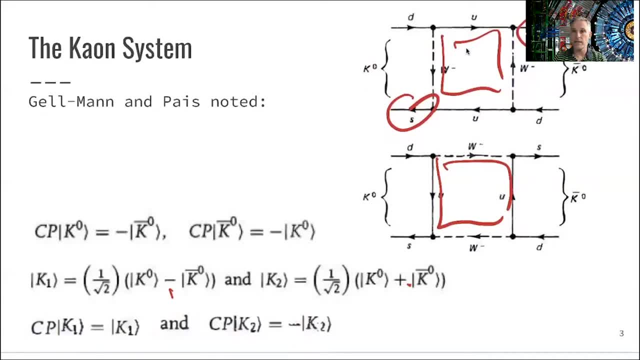 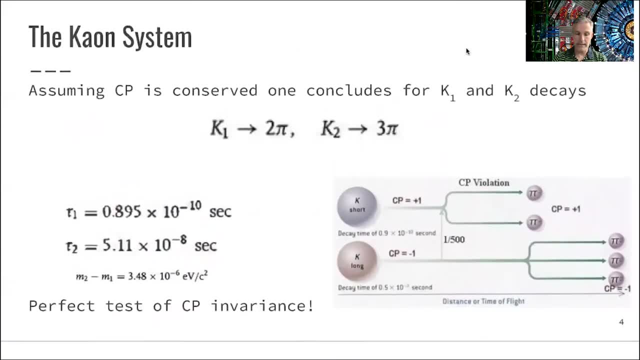 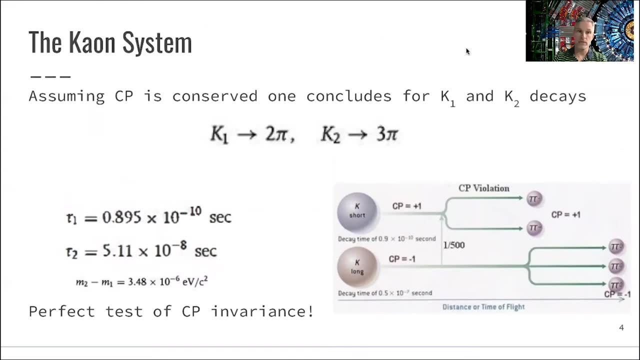 Good. So if you apply CP on the eigenstates, you find eigenvalues of 1 and minus 1.. It turns out that the lifetime of the k1 and the k2, those eigenstates is very different. One is 10 to the minus 10, and one is 5 times 10 to the minus. 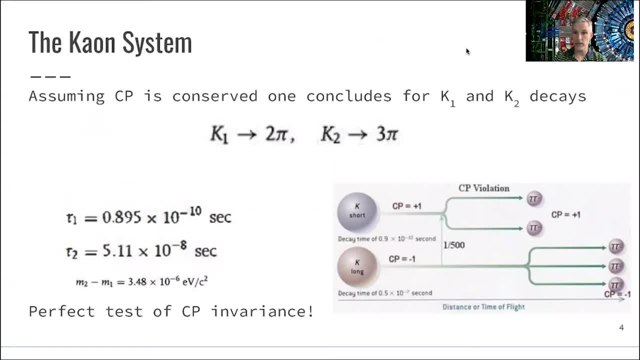 8. So The k1 decays much, much quicker than the k2.. So this then sets the stage to a test of CP violation. So what you're going to do is prepare a beam of k0s and let them decay. 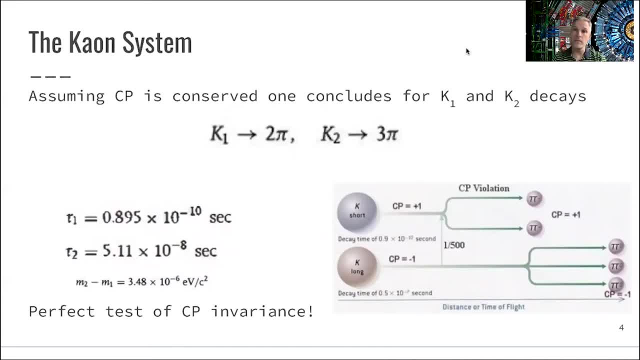 And only after some time you study the beam again, which then should be made up solely of k2s. So if you in that beam observe decays of the k2 into 2 pions, you know that there is an antiparticle. 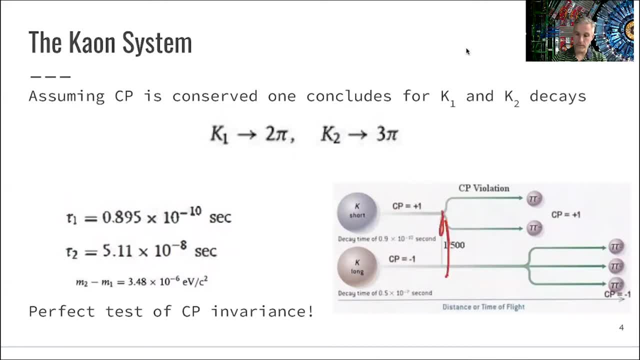 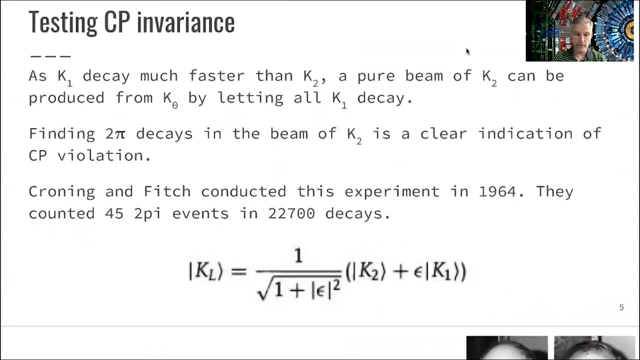 There is an admixture again which violates CP. So you have an admixture of k1s in a beam which should just be of k2s, So that mixture then will violate CP invariance, And exactly that was done. 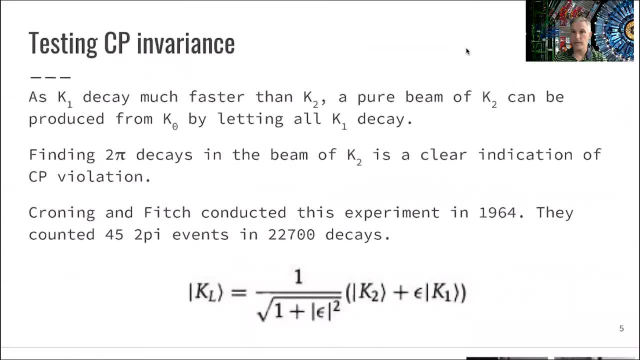 So Kroning and Fitch picked up this idea. They set up an experiment in which they produced kaons. They had them decay, And then they studied later in the beam whether or not they could find 2 pion decays. And they did indeed observe 42 or 45 pion decays, 2 pion decays. 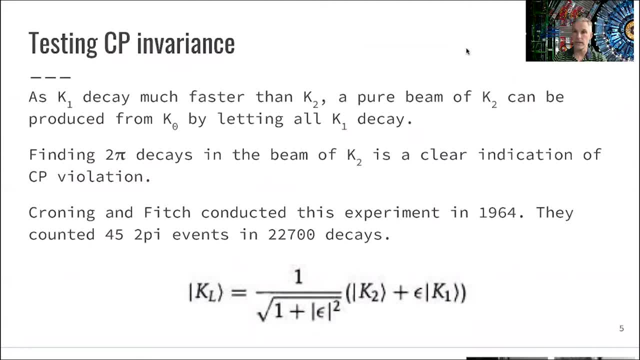 in a total of 22,700 decays. So that means that this k-long beam, the long-lived kaon beam, is actually an admixture of k2s with a small additional component of k1s. So here they observed. 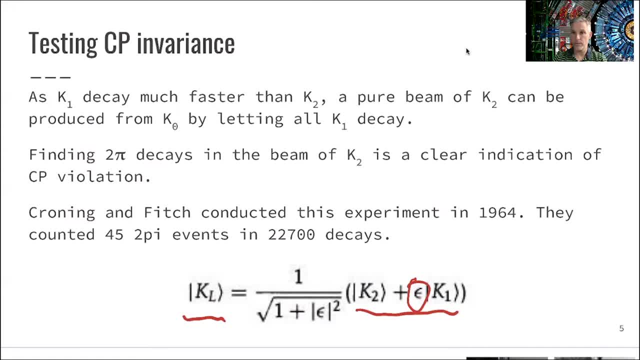 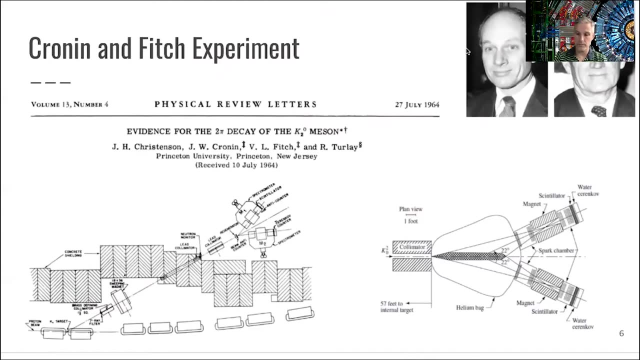 There was a pretty giant CP violation through the mixture of those states and this epsilon gives you the size of the strength of the CP violation. So here is a note of the paper. We'll have another discussion of this in class by student presentation: Kroning and Fitch here. 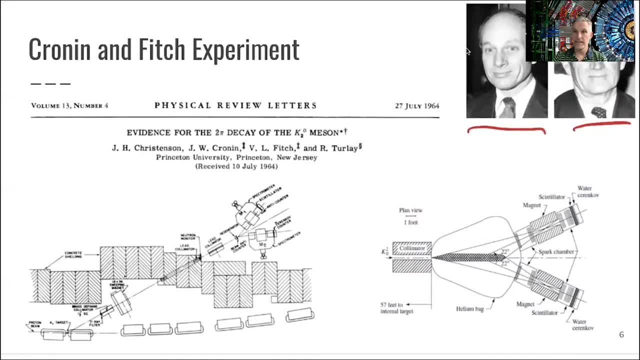 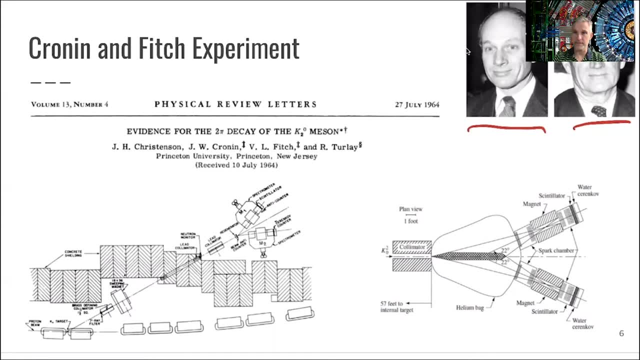 This is Kroning And this is Fitch. It turns out that Kroning is actually a student or was Fermi and also worked in Chicago, So that's quite an interesting family tree here, to which also Jerry Friedman belongs. Jerry Friedman is a retired faculty at MIT. 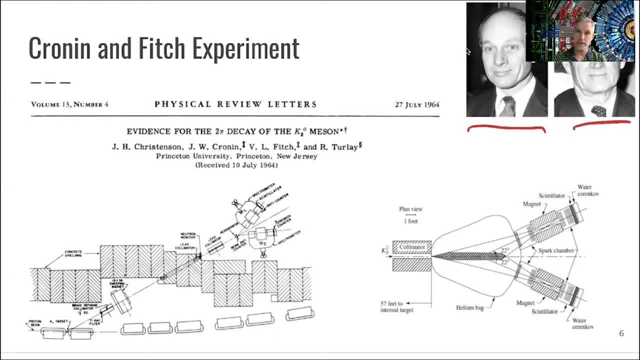 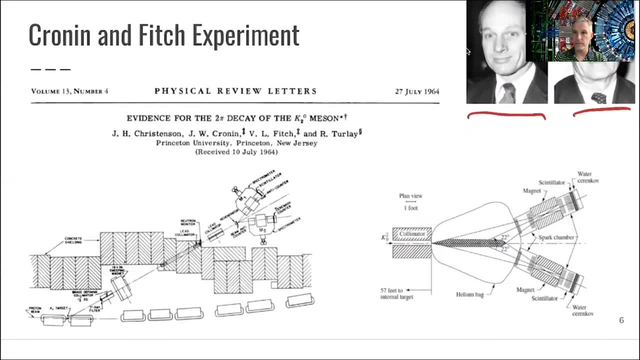 and discovered that protons are made out of quarks, So this is a very interesting family tree. If you have some time, you might be looking at this, But here's the experiment. So you take protons, You dump them into a beam. 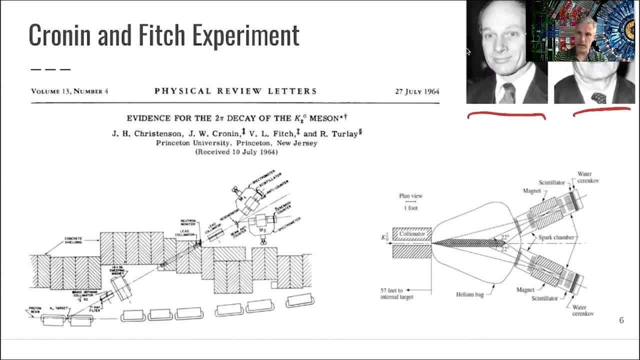 You try to, with this magnet, filter out a neutral component, get rid of all photons and then let this beam decay. And look in the spectrometer for decays of two photons. Here's a bigger picture of the same spectrometer, because this is a blow-up view of this. 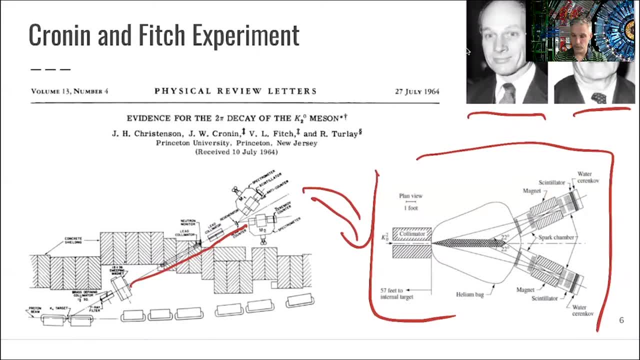 So you have your kaons, neutral kaons, coming in the K2s And then you look for two pion decays. The instrumentation and how we actually would do this is part of later discussion that we actually talk about detectors. 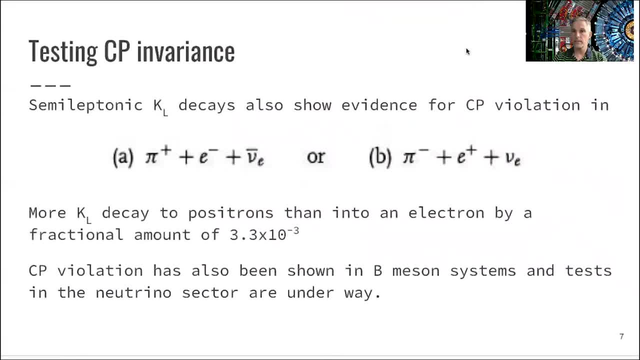 In more detail, All right. so we just saw that Cronin and Fitch observed CP violation in a mixture of states, But we can also observe CP violation in direct decays, And the classical example here is the case of the K-long and semileptonic decays. 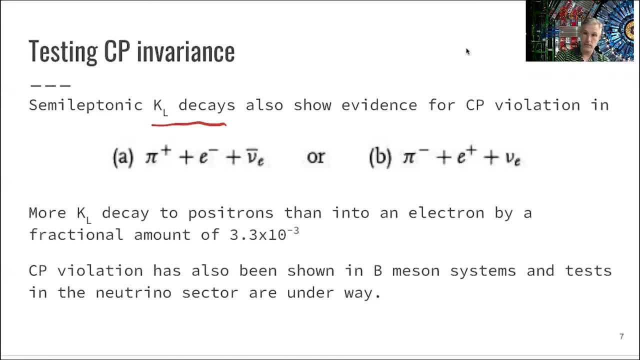 So semileptonic here means we have a decay of the K-long, the neutral particle, in a charged pion, an electron and an antineutrino, Or it might very well Also decay into a pi minus, a positron and a neutrino. 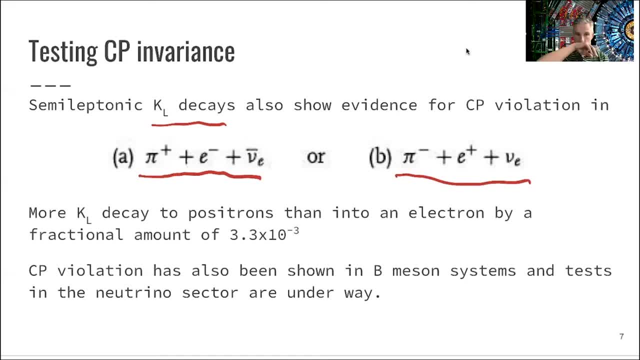 And it turns out, when you really count those events and perform a precise experiment, that the K-longs prefer decays to positrons over decays to electrons, And so the fractional amount of this imbalance is 3 times 10 to the minus 3.. 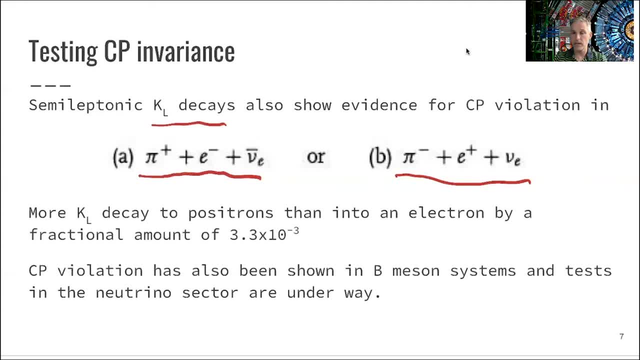 So this is a rather small effect again of CP violation here in direct decays. Since then CP violation has also been shown in the decay of B mesons And the program of studying B mesons is a big part of the LHC experiment at the LHC. 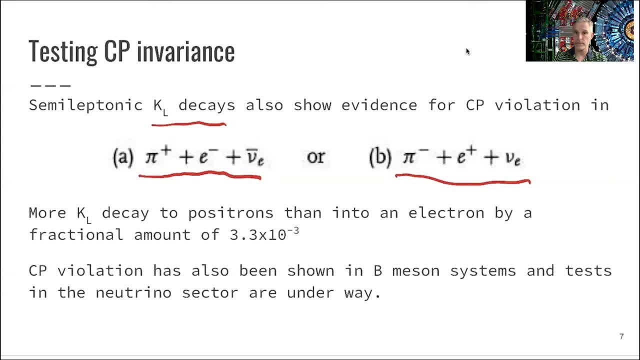 There's also experiments in Japan going on right now which study B mesons in order to learn further about B systems. Tests are also on the way- for those who listened to the colloquium on Monday- in the neutrino sector. So here we have a completed 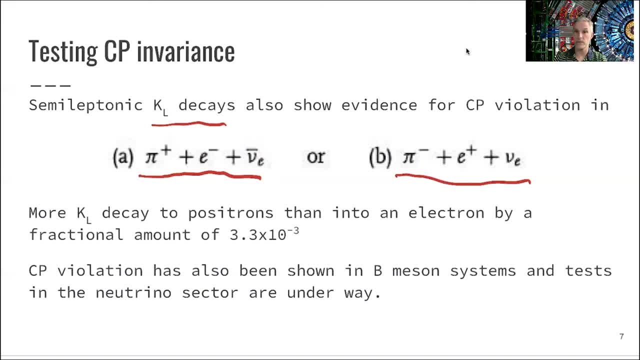 There are two different parts. so not quarks are involved in weak interaction, but neutrinos, And so the question is whether or not in that sector of physics, that sector of the standard model, is CP violation. Those are aspects we'll discuss later on when we talk. 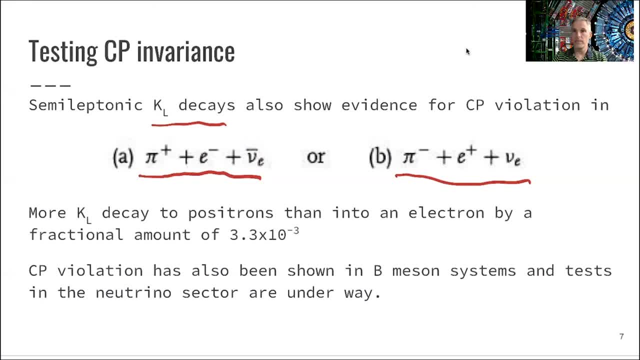 about neutrino specifically. Before I close, a few more remarks on the meta-anti-meta symmetry. One of the biggest mysteries in physics, I would claim, is the fact that we are even here to ask this question. So there is apparently more meta in the universe than anti-meta. 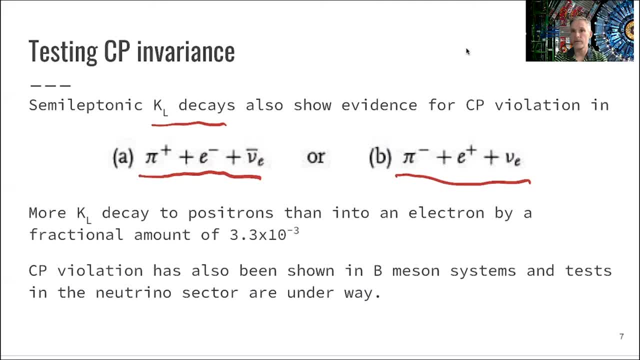 If you start from a Big Bang, there was this symmetry, And now we live in a universe which is dominated by meta. So how is this possible? So in 1967, Sakharov proposed that this is possible in a system where bar your number is violated. 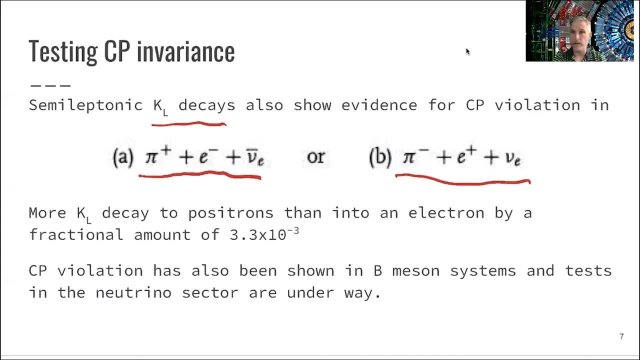 So this is almost a trivial. If you start from an equal number of baryons and antibaryons, the sum is then 0. The baryon number is 0 of this system And you end up in a system which is dominated by baryons. 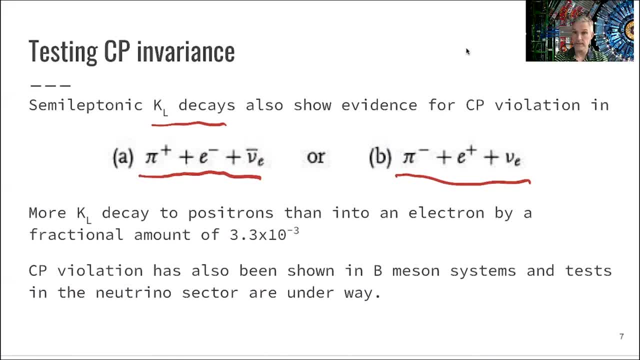 then baryon number needs to be violated, But there's also the need of CP violation in this. So we just saw that this is realized in nature, But the amount of CP violation we observe in this system I just discussed it's not sufficient to explain. 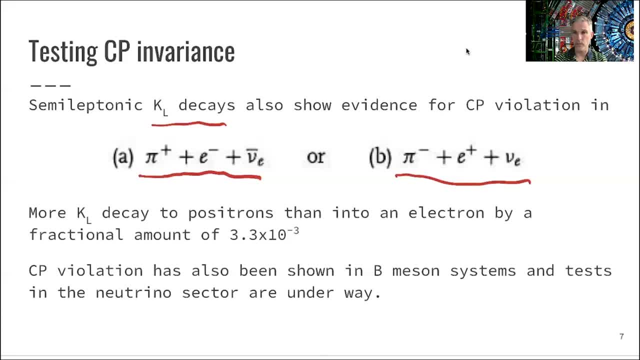 the meta-anti-meta symmetry. It's meta-symmetry we observe in nature. So there is more to be found, There is new physics to be looked for in CP violation, on this overall question, And there's also a need for the actions. 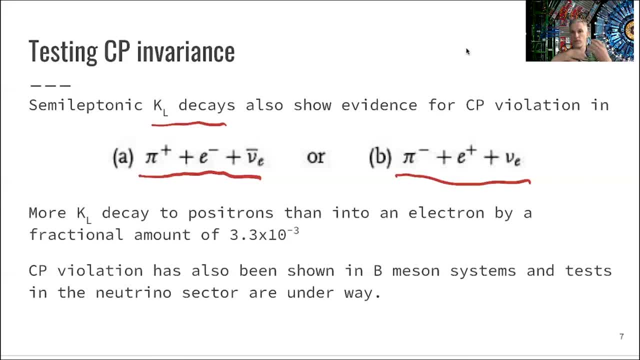 to be out of equilibrium, meaning that you don't revert the processes as you go forward. Yet another point of discussion, which I will not go into much detail in this lecture, is that you know our quantum field theory, which describes the standard model. 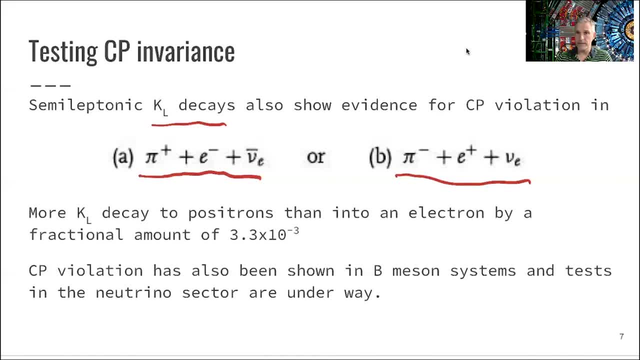 and describes the interaction of particles is invariant under CPT transformations. That means that if CP is violated, time reversal cannot be a symmetry. So meaning going backwards and forward in time is not symmetric, And you can test this. You can design experiments which test the effect. 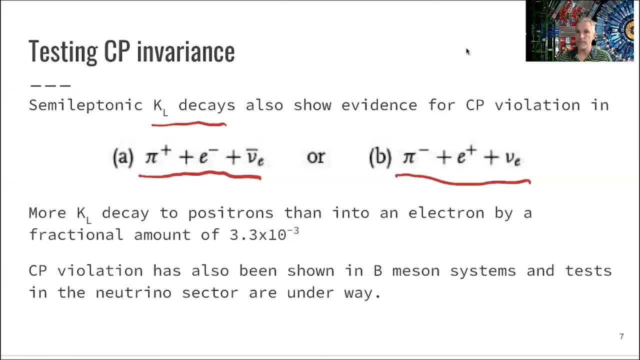 You can also design experiments which test CPT directly. So those are all interesting questions, but we will not go into any of those in this lecture. We will, however, come back to understanding the origin of CP violation in the standard model when we talk in more detail. about the weak interaction.